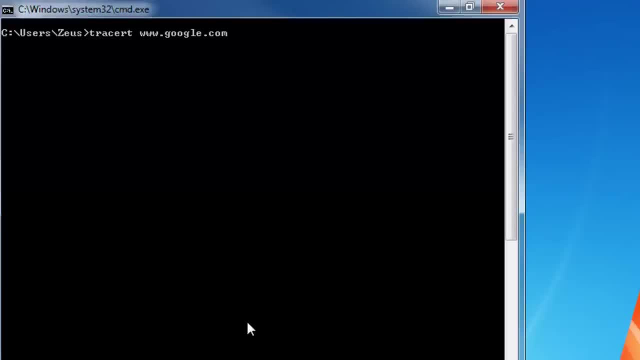 complete list of the route we are going to take to reach Googlecom, and I'm going to explain this to you once the trace is complete. So let's press enter to start the trace and I'm going to wait for the trace to complete and then analyze the results really quick. 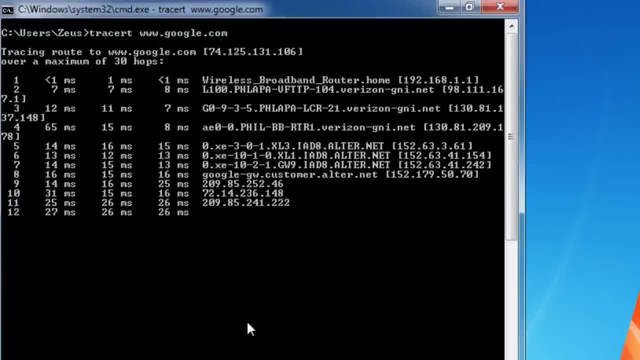 wwwgooglecom. Okay, so the trace is complete. Let's see what's going on here Now. anytime you go online wwwgooglecom, wwwgooglecom- to anywhere other than your own local area network, what you guys usually think is you type in wwwgooglecom. 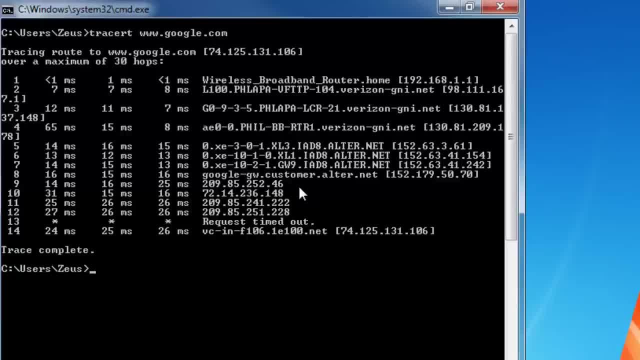 and boom, Google just shows up, right. what actually happens in the background is you travel through hundreds of routers before you reach your destination. sometimes less than a hundred, but mostly it's a large number. okay, and the trace RT actually prints every single one of the routers that you hit. 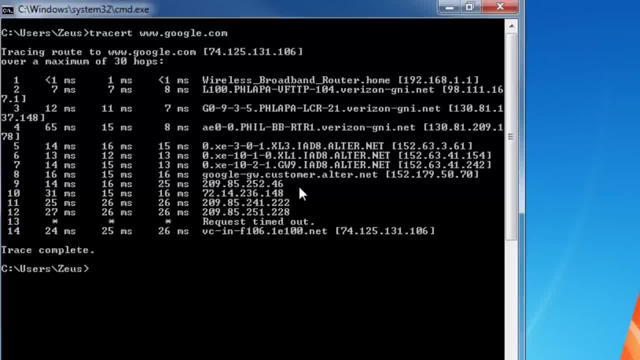 on your way to your destination. okay, that's how the internet works. the internet is a network of hundreds of thousands of millions of routers that you route, get routed through to reach a destination. okay, so let's take a look at what happened over here. so what I did was I want to go to googlecom. okay, so it's saying here: 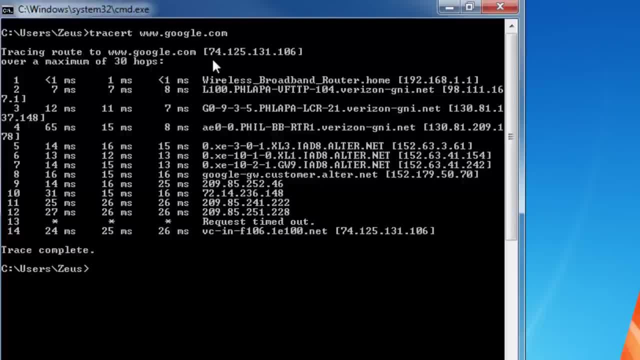 tracing route to wwwgooglecom. it gives you the IP address of googlecom and it starts the route on the tracing right over here at number one. so the first thing it hits is my own wireless broadband router in my home. okay, so this is my router. that's the. 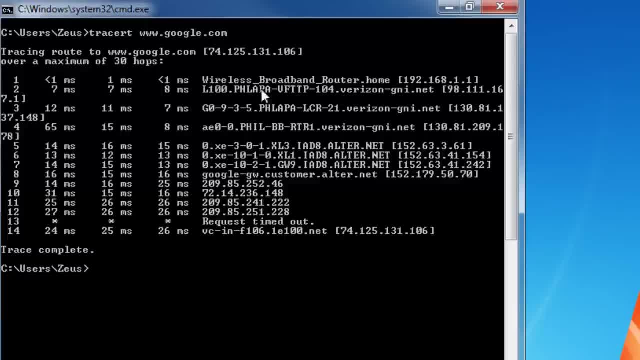 first router we hit. the second router it hits is a Verizon router. so if you look over here it says verizon, blah blah, blah dot net. so I do go through the ISP called Verizon, so it is natural that it hit the Verizon router. now the third router is again a Verizon router and then it goes through different routers. 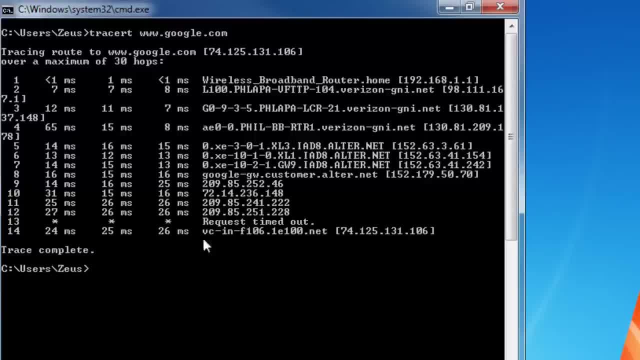 until it finally hits the verizon router. wny reaches googlecom. but if you look at this total numbers over here, the final number is number 14. so it took 14 routers for me to reach googlecom. and also I just wanted you know that this is also called fourteen hops. so if I say 14 routers, 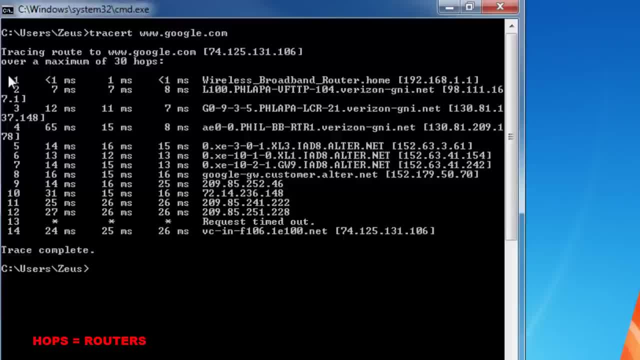 it's the same as fourteen hops, so it took me fourteen hops to reach google dot come and also it. let you know that the highest number is always 14 hops faster than the highest number. devices editing schedule users and can control the speed for the system. sometimes it takes aεν key to write down your 210�MHz ratio & árt». 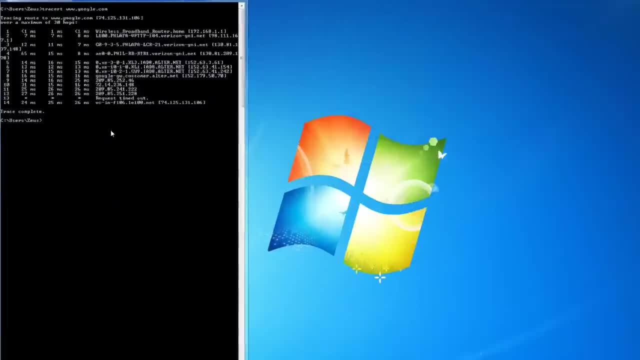 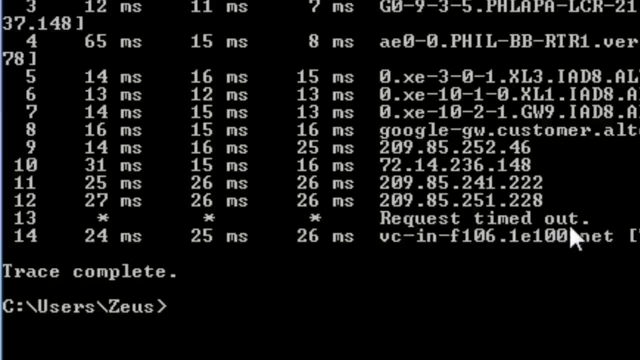 there are some routers out there in the world that do not let you run a trace RT on them. so if you look at number 13, the request was timed out. either this router dropped the packet, so it does not accept trace RT packets, or this router was not working, so we were directed to the final. 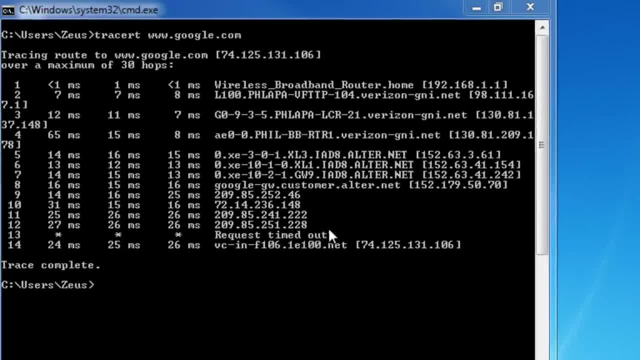 router number 14, all righty. so sometimes the router does not work and sometimes it drops the packet. it silently drops the packet, doesn't tell you why. you just have to make a guess over there. but um, so how can we use this as a diagnostic utility? let's say you were going to a website. 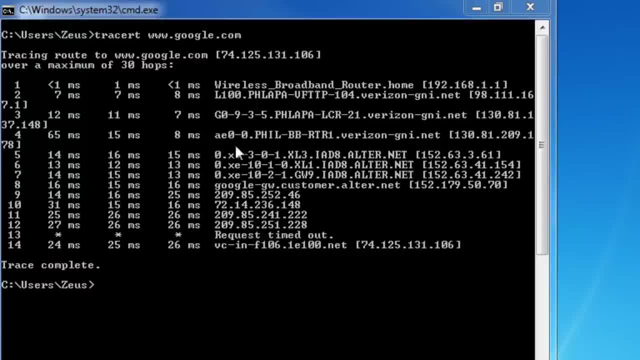 let's say, googlecom is working for you right now. that means you're going to see this whole trace all the way. now, if googlecom goes down- okay, or if your ISP goes down- what's going to happen is at number two, here in your ISP's router, the trace is going to stop. 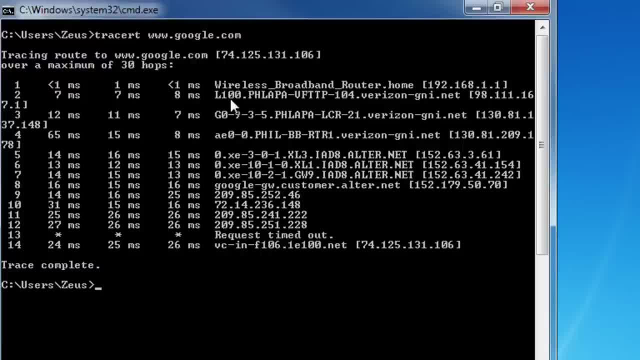 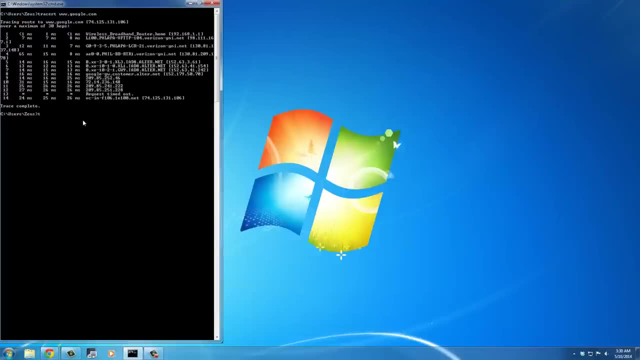 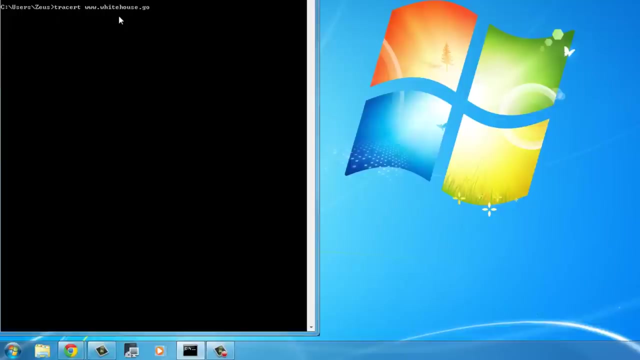 it's going to go no further than your verizon ISP. then you can call verizon and you can tell them. hey, listen, I was trying to reach googlecom, which your routers are not routing the packages, so I can go to googlecom. okay, let me run one one more trace: RT: wwwwhitehousegov. 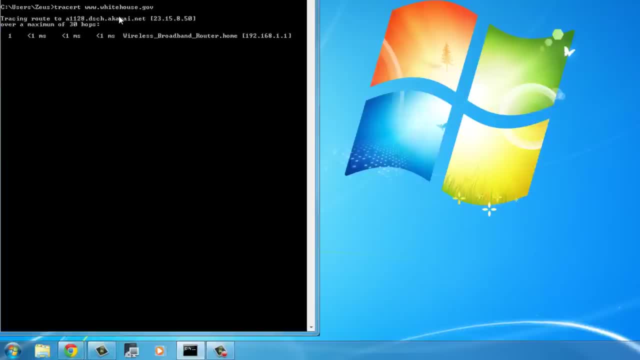 is it gov? yeah, gov. so are going to be routed to the White House's website, And this was fairly quickly. So the first router is my own wireless broadband router, just like on the top here. The second one is the Verizon router, just like the one up here, And then it's going to get routed through a bunch of 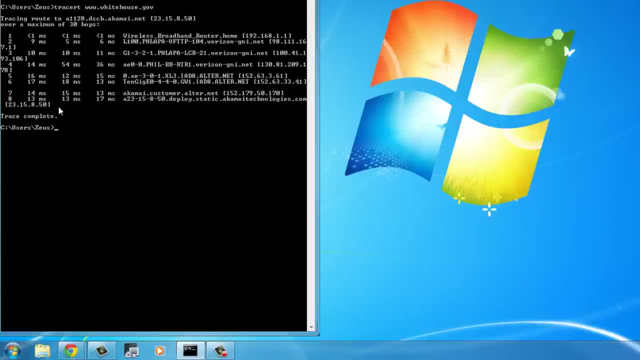 different routers until it finally reaches the destination. So if you look over here, we went through 1,, 2,, 3,, 4,, 5,, 6,, 7, 8 different routers to reach whitehousegov, which makes sense because 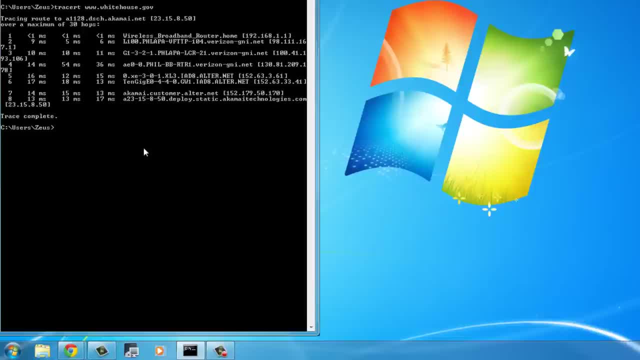 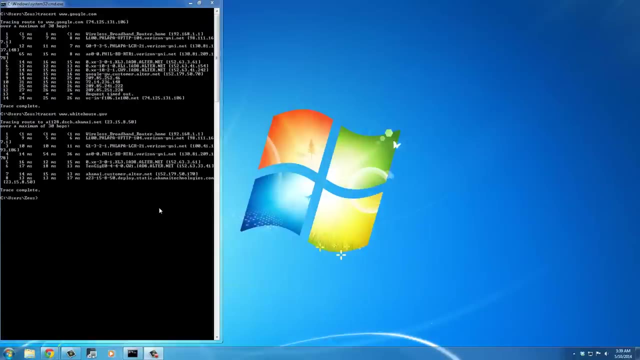 I live in PA and White House is down in Washington, So it makes sense that it only took me eight routers to get to whitehousegov, as in, where Google took me 14 hops, And we know that Google is not in this East Coast. All right, now that we have two trace RTs over here, let's 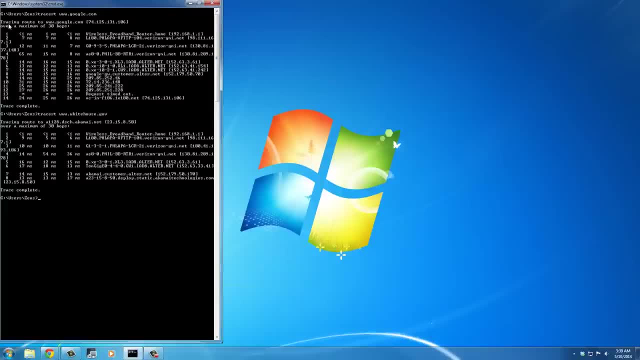 look at the next one. So the first router is my own wireless broadband router, just like on the look at a look. look at something over here that's interesting. so tracing it's over here. it says tracing route to wwwgooglecom over a maximum of 30 hops. 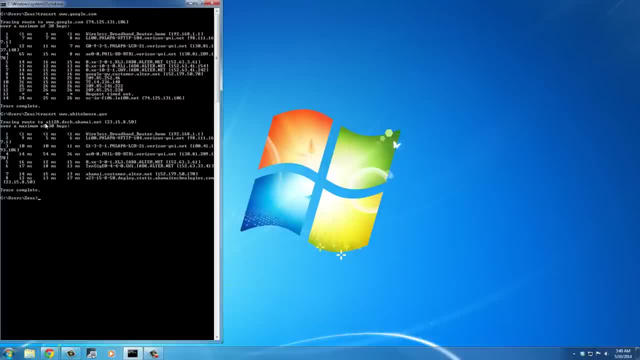 okay. at the bottom here says tracing route to whitehousegov over a maximum of 30 hops. so what is this maximum of 30 hops? what that stands for is, if you hit more than 30 routers to reach a destination, the trace route command stops at the 30th hop. okay, so the maximum amount of hops you can trace by. 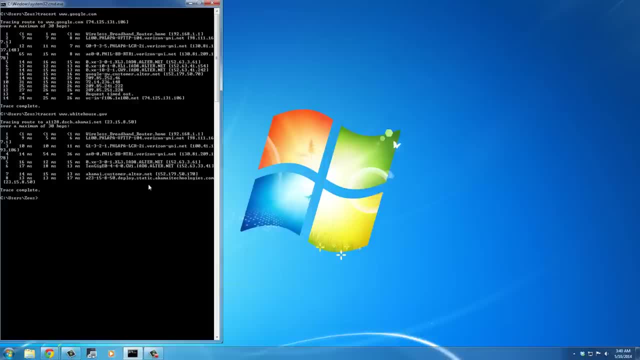 default is set to be 30 period and then on, what you can do is you can use a parameter under the trace RT command to actually change the number of hops you want to travel. so let me show you how to do that really quick, okay, so the the 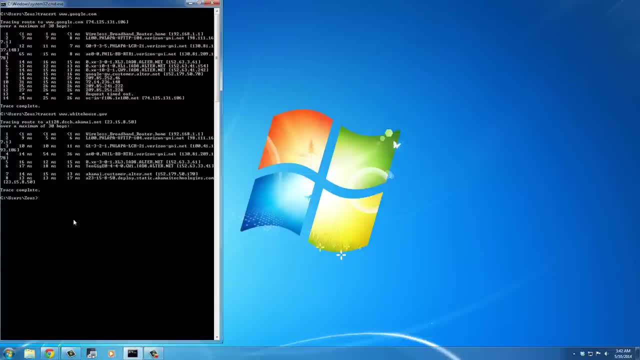 parameter that we're going to use is called minus H. so you type in trace RT, you say minus H and then you define the maximum amount of hops you are willing to take. you can put in 60, you can put in a hundred before the trace terminates. let's do five and let's run this on the 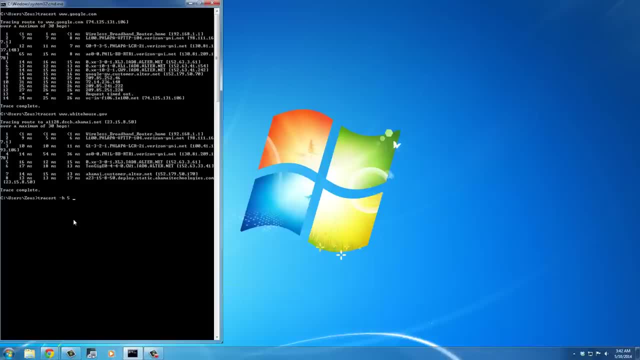 whitehousegov. so I can show you how it's going to terminate after the fifth hop. so, whitehousegov, let's enter. okay, as you can see, the trace is complete. so on the first spot, we took eight hops to reach whitehousegov. on this one over here with the minus H. 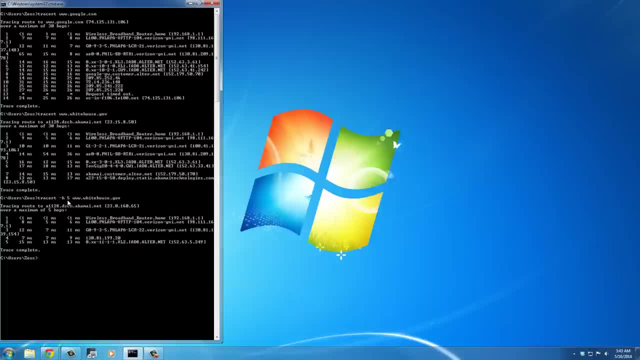 parameter. we define the maximum hops before the trace RT terminates to be five. so the trace was complete in five. let's do one more. so trace RT minus H. let's just do four. let's do three: wwwgooglecom. so this should terminate on the third hop. 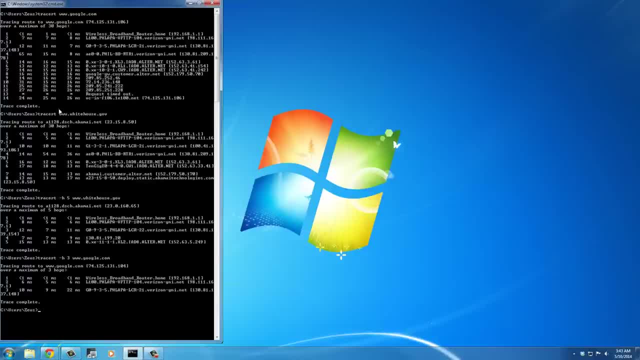 boom, it's over. okay, so you can actually change this number. this is just a default number of 30 hops. you can also go beyond thirty to a hundred hops. all righty, all right. so let me just clear the screen really quick. CLS to clear the. 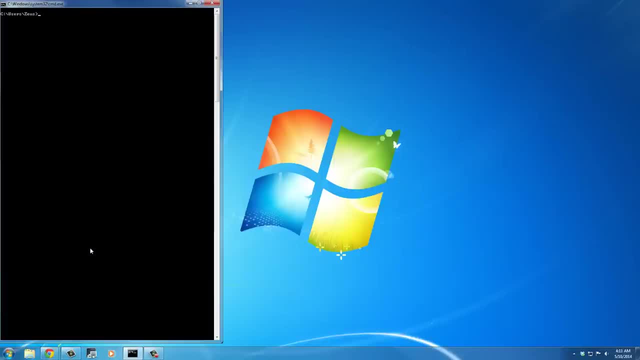 screen and type in one more command. well, not a command, but a help tool. so if you type in trace RT and then do slash question mark, you will get a list of all the parameters that you can use with the trace RT command, and not all of them are that important, but the one I showed you. 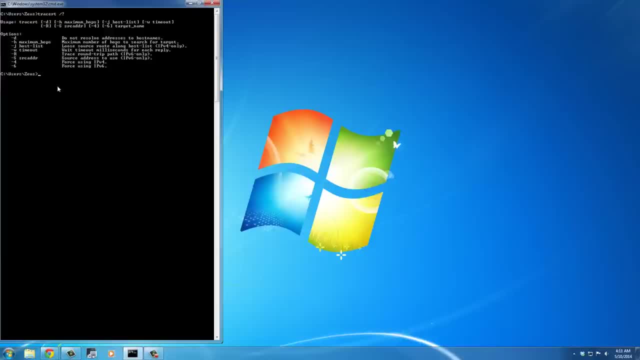 was important and you can check the others yourself. so just remember, with trace, RT is a diagnostic tool because it traces your packets okay. so if you're trying to reach googlecom but you can't reach it, you are able to find where is the failure happening. so if it's failing in, 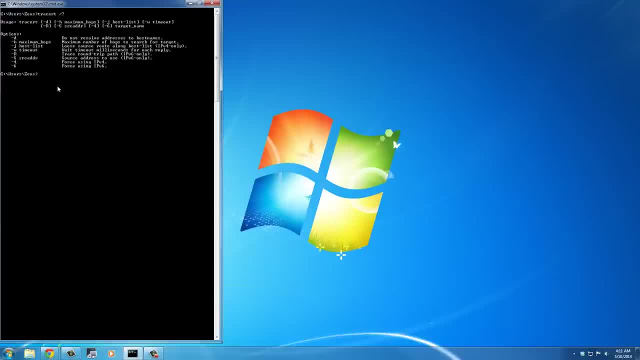 the second hop. that means your ISP has a problem. if it is failing all the way in the middle somewhere, you know it is not your ISP, it is somebody else. not much you can do about it, but it is still information. and then you can also gather some miscellaneous information. I'll give you an. 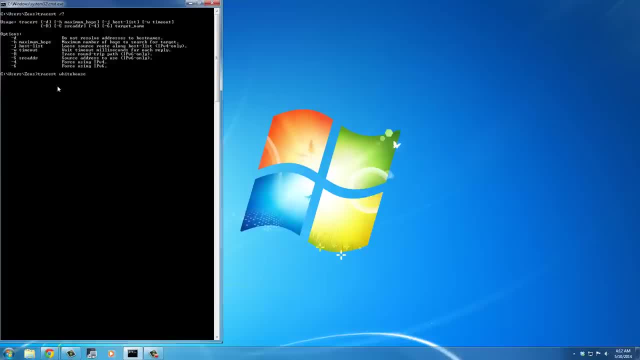 example. so let's do a trace: RT, whitehousegov- okay, and what I'm gonna do is I'm gonna press ENTER and if you look at these names carefully, there are some descriptive qualities to these names. so as I come closer to white house- which is, as you come closer to number eight, the last hop- you start saying: seeing this: 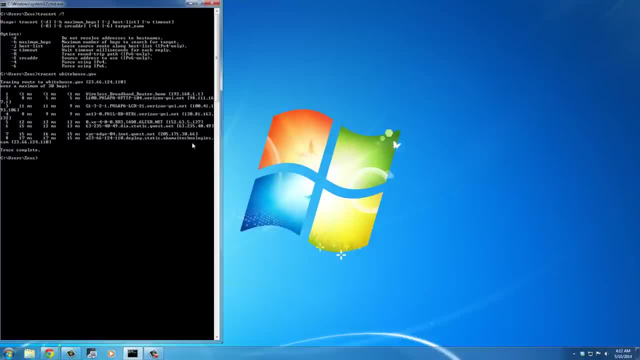 thing called Akamai technologies. okay, so I'm going to go ahead and go ahead and look at these names. so basically, you can deduce by looking at this that the white house actually has business dealings with Akamai technologies. now, when you go to google and you type in Akamai technologies, it comes to be that